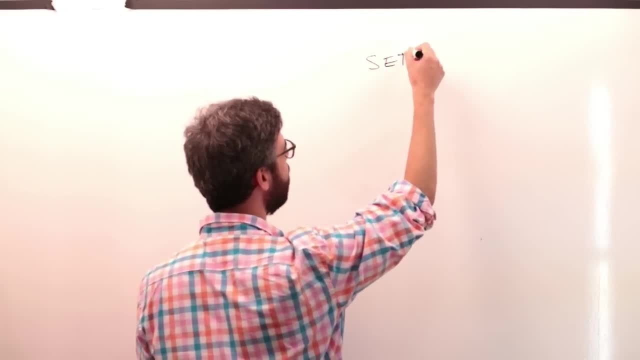 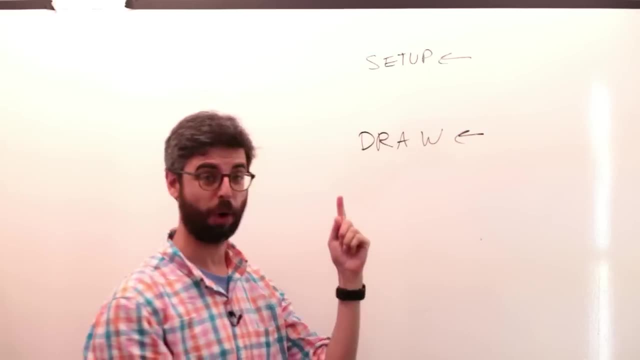 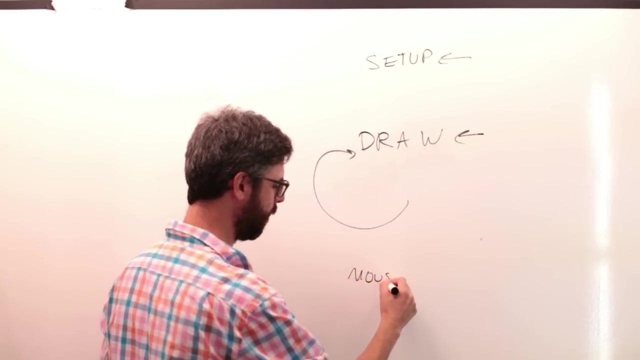 The only path we really have right now is starting in setup. That's the first thing that happens, Moving on to draw and looping over and over again. Draw, repeats over and over again. We saw that you have these event functions, Like there was also the event function mouse pressed. 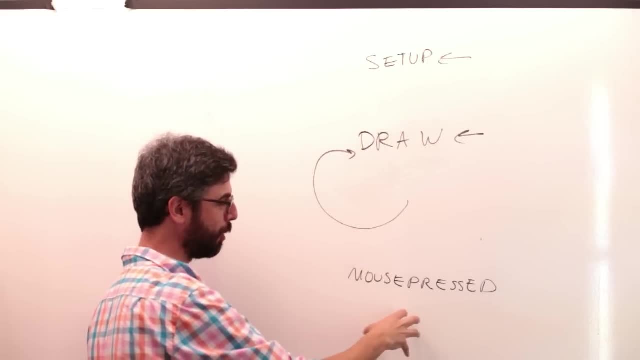 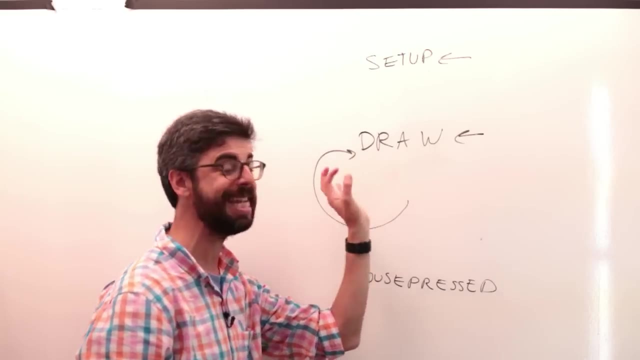 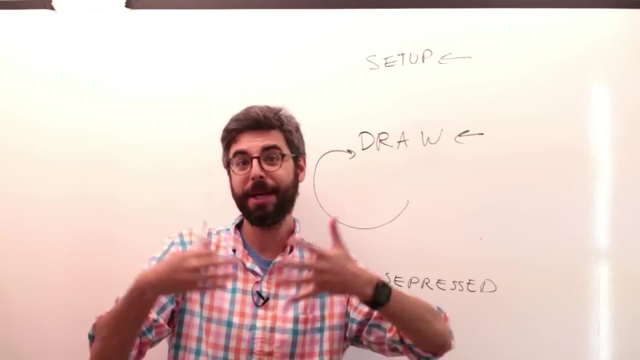 So if you clicked the mouse, the code would take a break from draw, go execute something down here and continue and draw again. But now I want to ask the question: how can the code execute differently each time through draw? So one time through draw it might draw a purple circle And the next time through draw it might draw a pink circle. 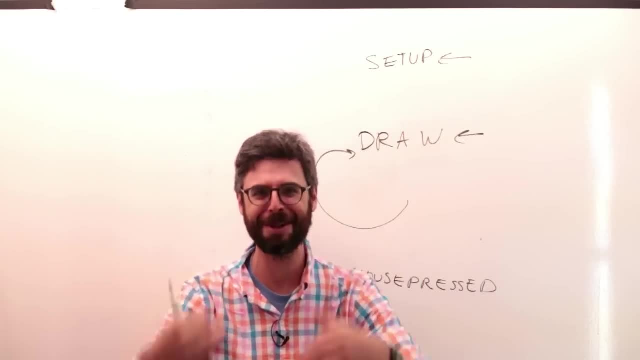 And, in fact, this I would like to be the first example that I make in this particular video. I don't know if I can get purple in here, I don't know if I can get purple and pink- just right, But I want to have a circle that's drawn with two different colors, based on something that the user is doing. 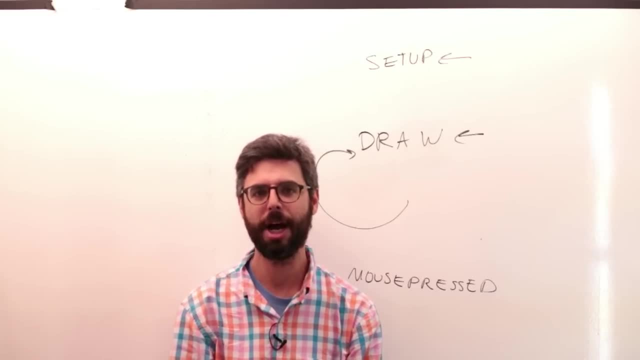 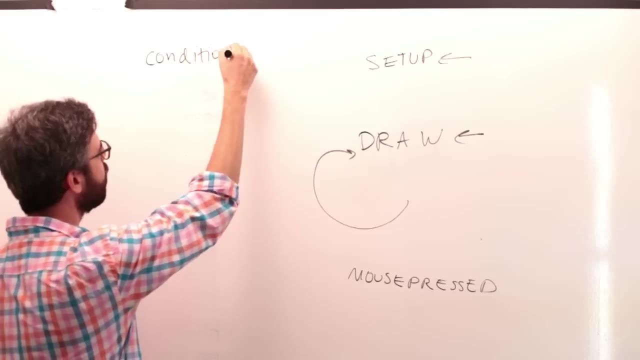 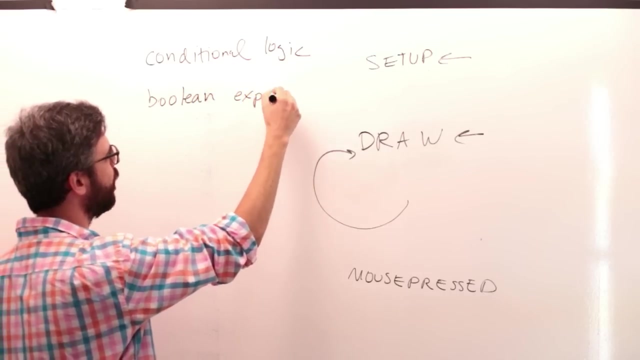 Perhaps where the user is positioning the mouse would be a good place to start. So in order to do this, we need to learn about conditional logic. Another sort of term we can think of in this case is Boolean expression, Boolean logic from the mathematician logician. 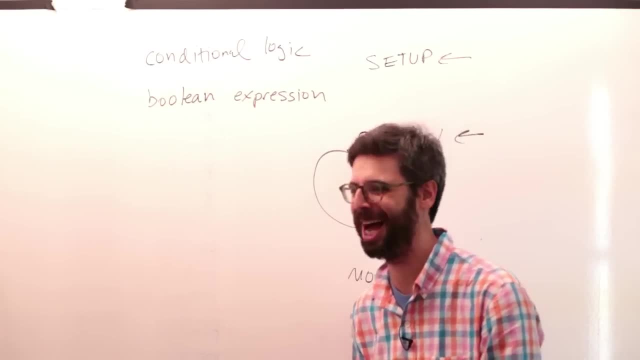 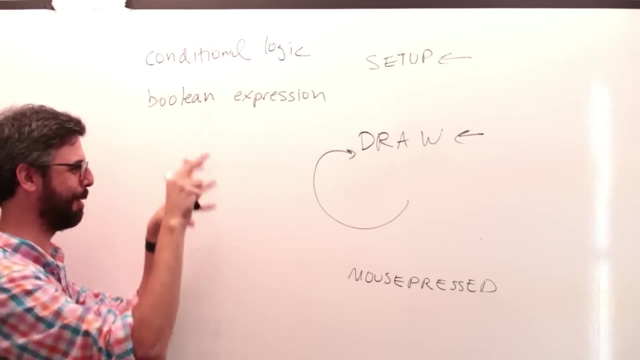 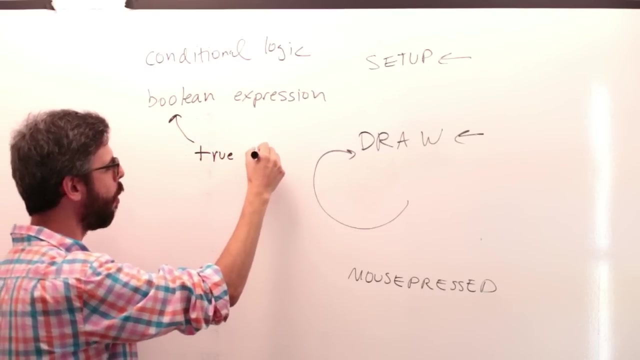 George Boulos, which I'm probably not getting right. Internet will correct me. I assume I'll dub this over or put some sort of like pop-up thing, I don't know, whatever fancy thing that works here. So Boolean. the word Boolean indicates that something is true or false. 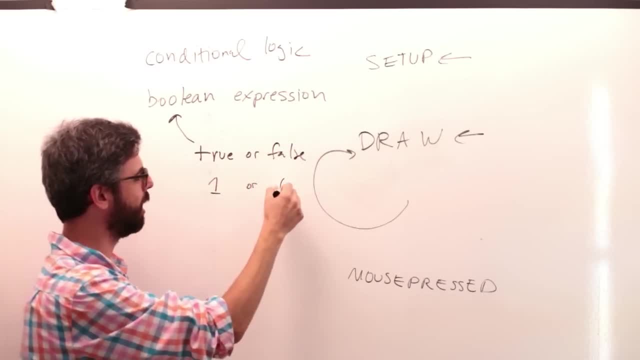 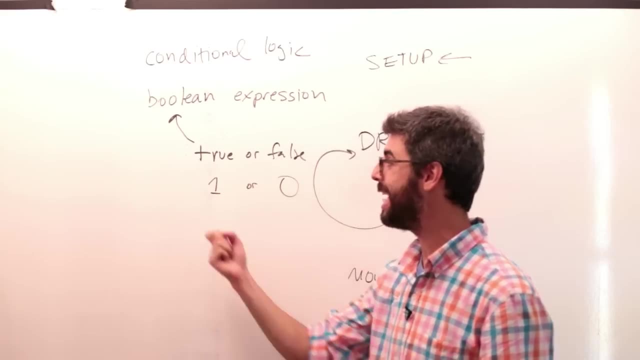 This is often also thought of as 1 or 0.. 0 being false, 1 being true. And what I'm going to show you how to write is an expression that says: if something is true, do this code. If something is not true, don't do this code. 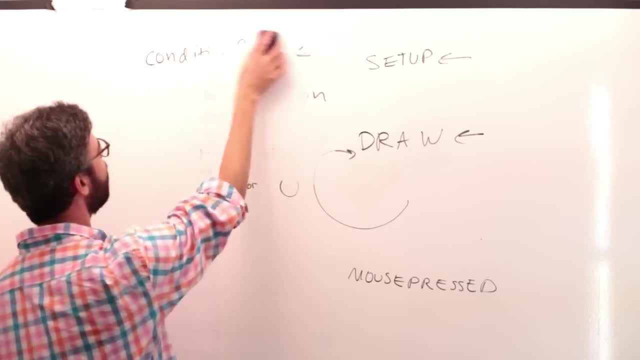 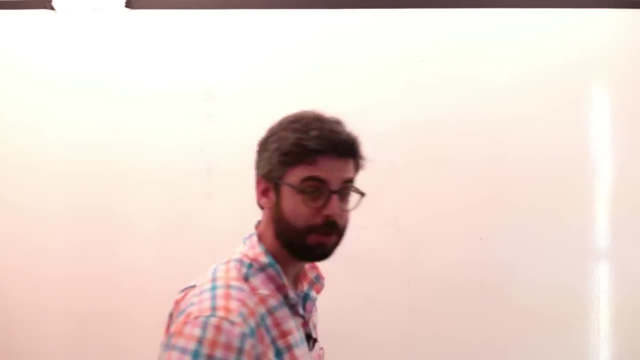 So let's think about how the kinds of things, the kinds of Boolean expressions that might evaluate to true or false. So I'm going to give you a Boolean expression right now and in your mind you will think about whether it's true or false. 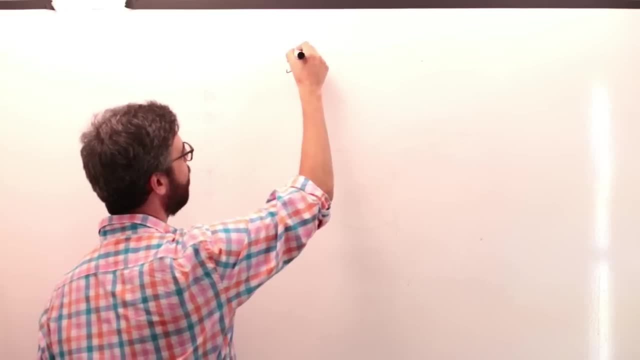 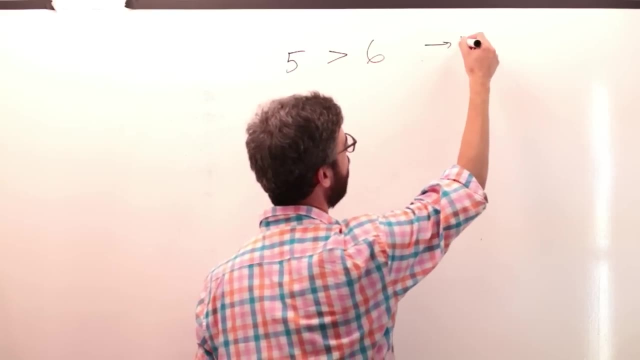 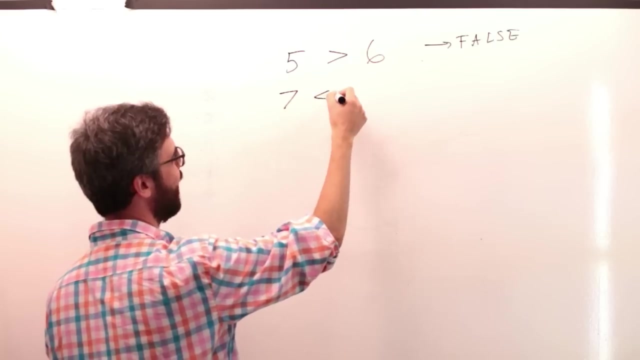 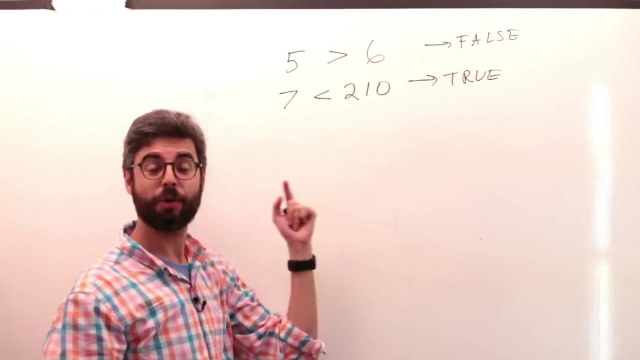 and hopefully this will be a rather easy one: 5 is greater than 6.. This is not true. This evaluates to false. There's another one: 7 is less than 210.. This is true. So you can see, I'm starting by creating these Boolean expressions. 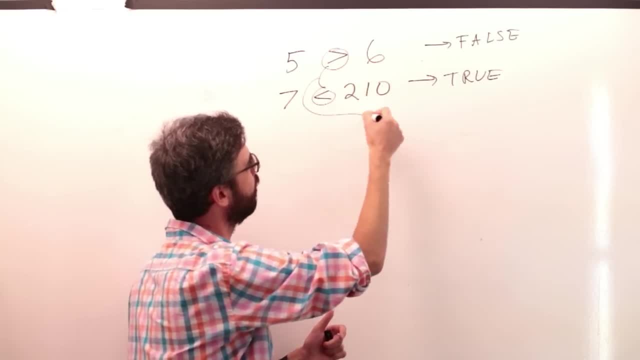 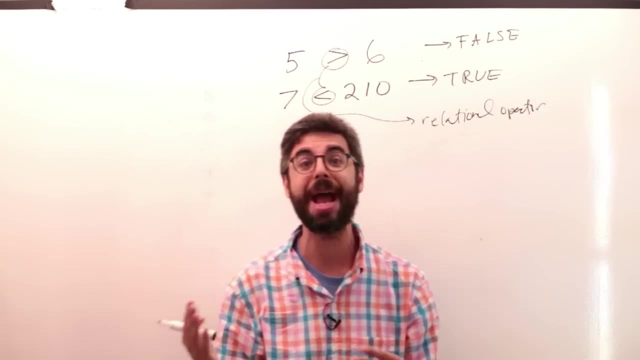 using something called a relational operator. A relational operator It's an operator that is going that, in this case, is going to compare two numbers. There's lots of ways eventually in code that you'll see that you can have something that's true or false. 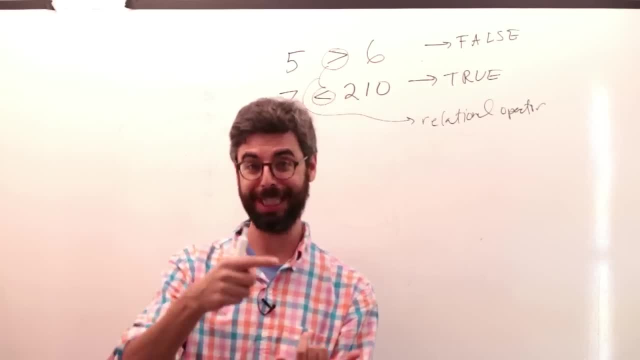 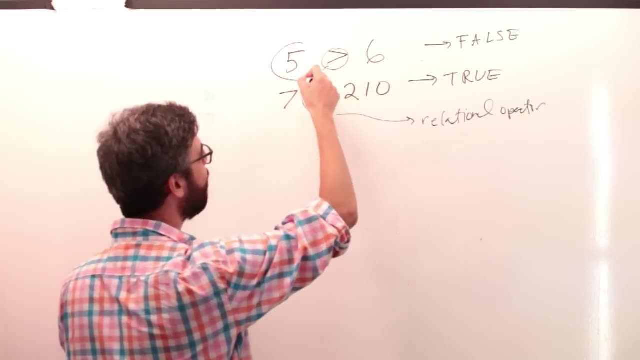 But a good way to start is just comparing numbers. Are these numbers equal? Is one number bigger than the other one, Or is one number less than the other one? So, now that we have this idea of how we can create a Boolean expression, 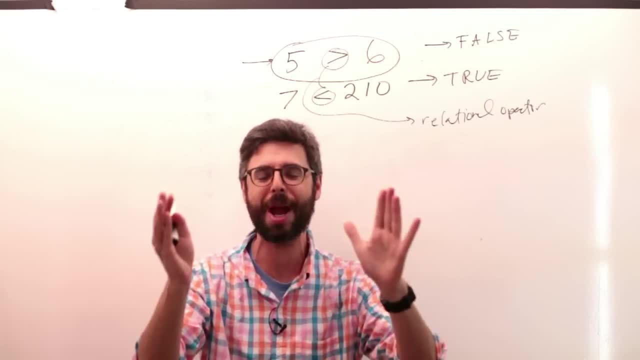 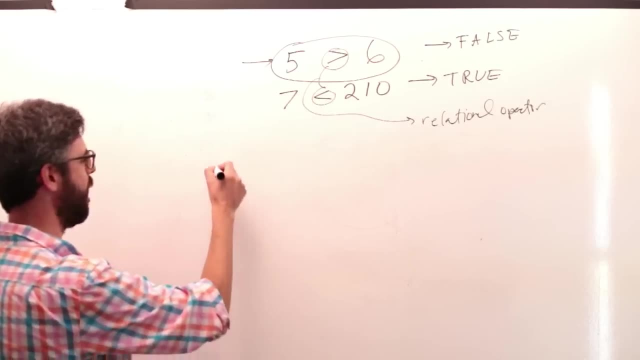 a mathematical operation that evaluates to either only two answers: true or false. we can learn the syntax for writing that statement into our code, And this is how the syntax works. If we've got a word in the English language, if that means exactly what it says. 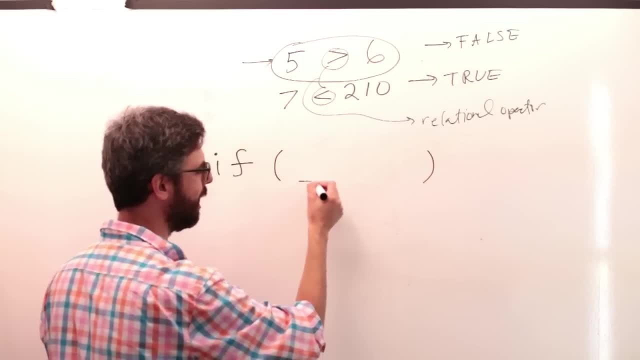 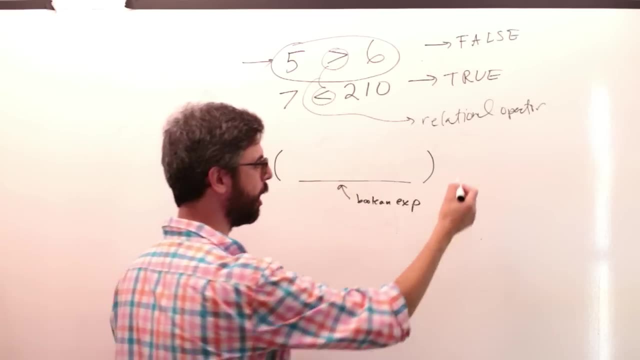 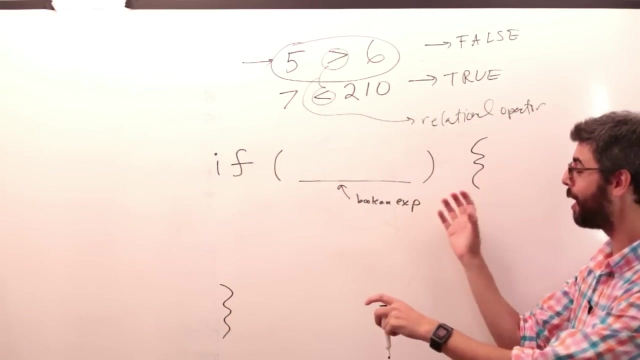 if some Boolean expression that is inside parentheses, this is our Boolean expression. if Boolean expression open curly bracket, close curly bracket, So we've created another block of code. This is a block of code with a beginning or an end, just like setup and draw are blocks of code. 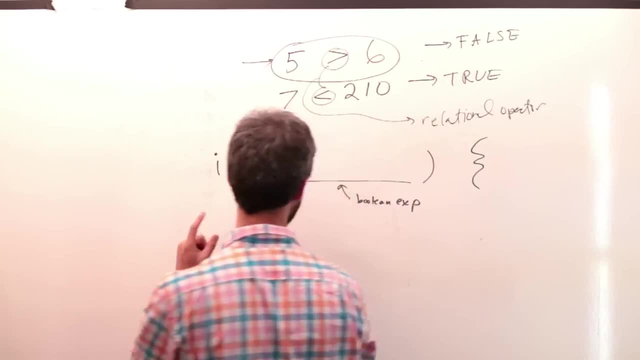 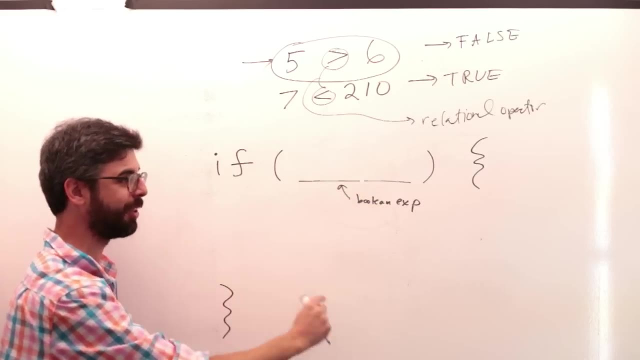 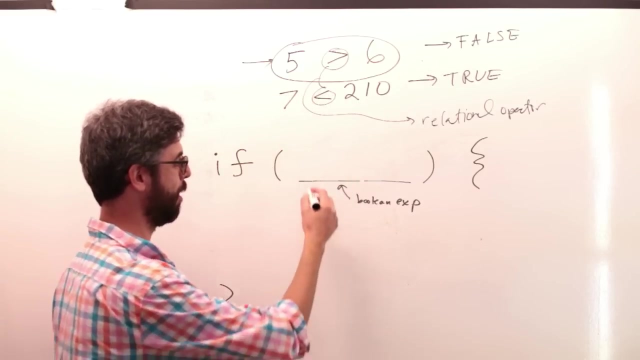 With beginning and ends. And the key thing here is: if this Boolean expression evaluates to true, then the code here should be executed. If this Boolean expression evaluates to false, then the code here should not be executed. So let's say, I write something like: 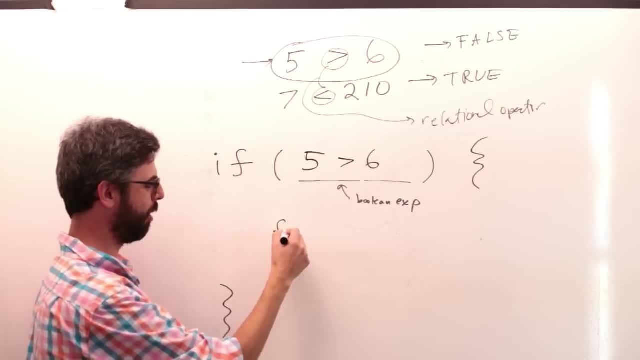 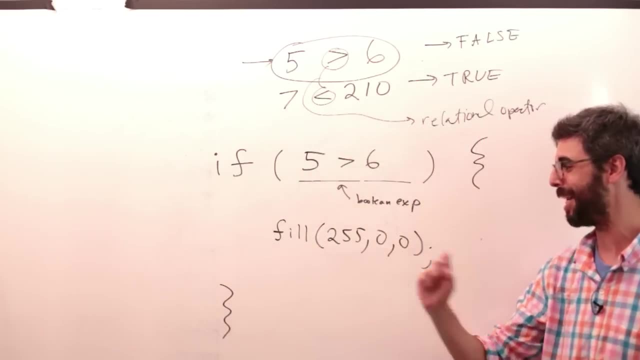 if 5 is greater than 6, fill 25500.. So, only ever, if 5 is greater than 6, should you set a red color. Now, if you're thinking about this piece of code here, you're realizing this is. 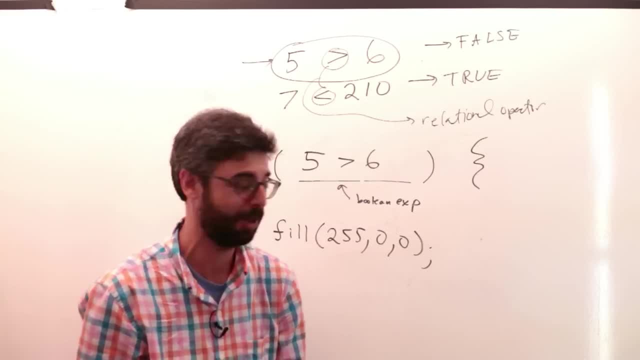 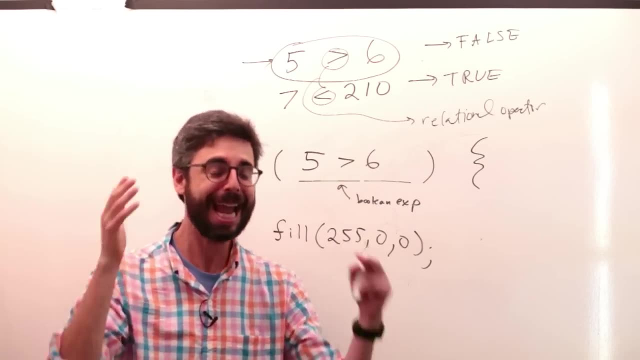 what I've created in this scenario is kind of ridiculous and useless in a way, Like 5, no matter how much we try over and over and over again, 5 is never going to be greater than 6. Ever, I can't. I mean, maybe there'll be another universe. 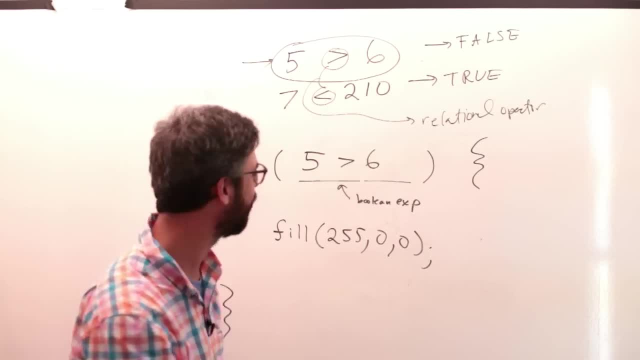 or a parallel universe or some other kind of wormhole thing we go through and 5 will be greater than 6.. But right now, in this room where I am under these very hot lights, that's making me feel a little faint for a second. 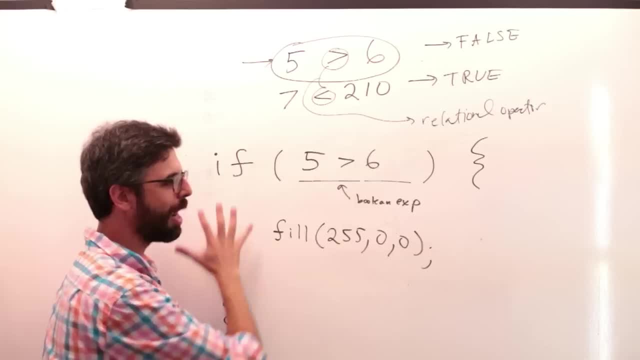 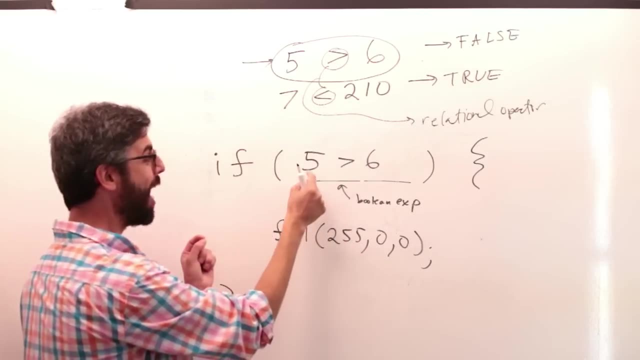 5 is not greater than 6.. So you can see, while this is the correct syntax, this is showing us the idea here- this doesn't really make any sense. The point of what I'm trying to show you is that if a variable is part of this Boolean expression, 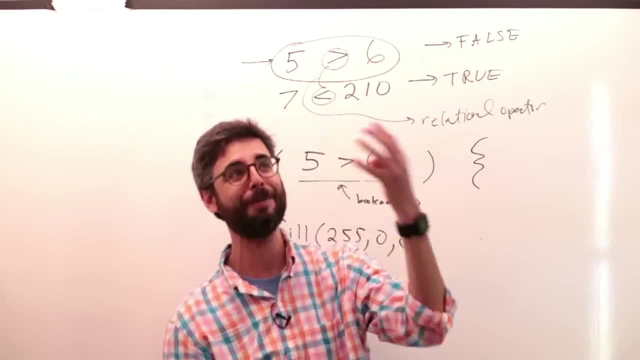 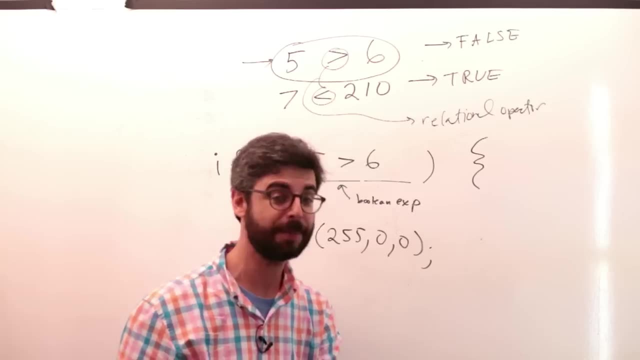 a variable has different values at different times of the day and different moments, depending on what other things are happening in the code, then that variable might sometimes be greater than 6, or might sometimes not be greater than 6., And so we can change this idea. 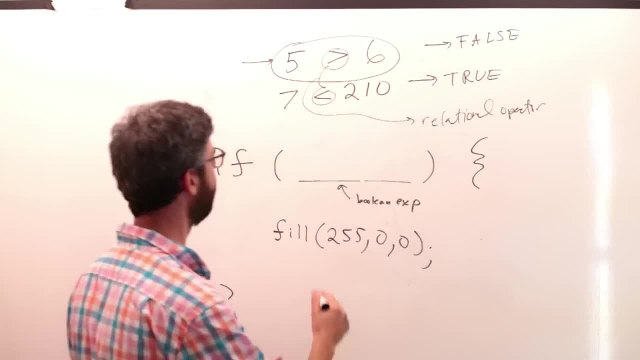 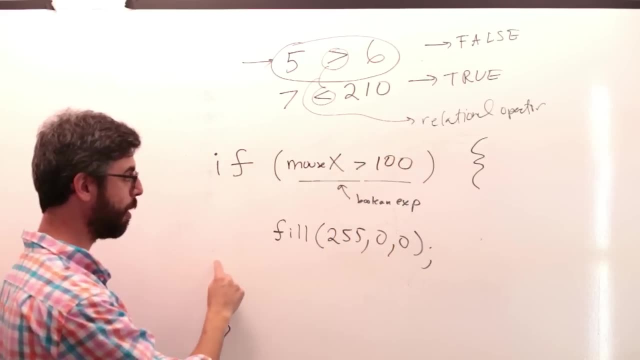 of this expression to say something like if mouseX is greater than 100. So now, as the user is moving the mouse, it's not greater than 100, it's not greater than 100, it is greater than 100. So this code, even though it's sitting there, 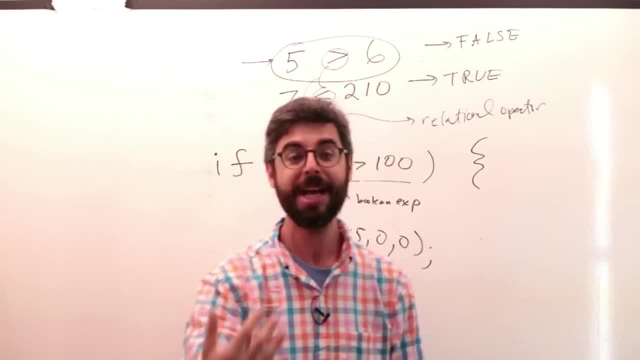 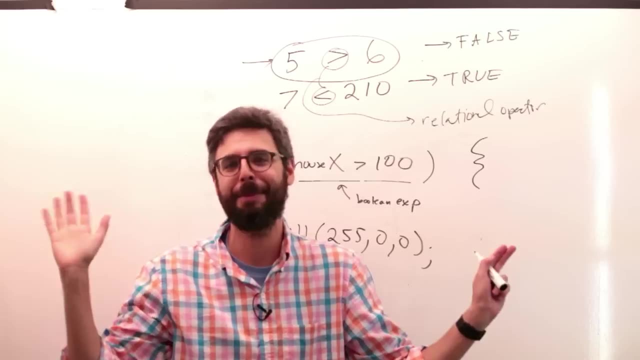 in the draw loop. I haven't put it there yet, but that's where it will live. this code will not necessarily be executed. In fact, you could run the program if the mouse never goes past 100, that code will never happen. 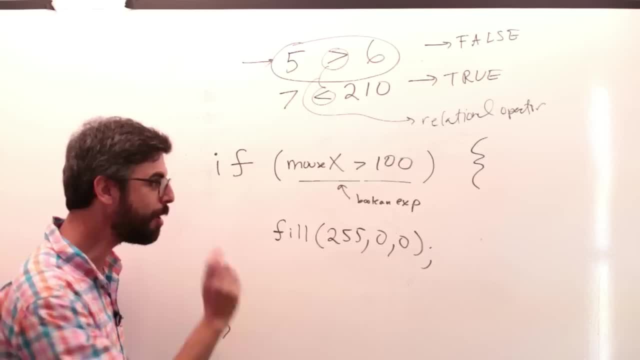 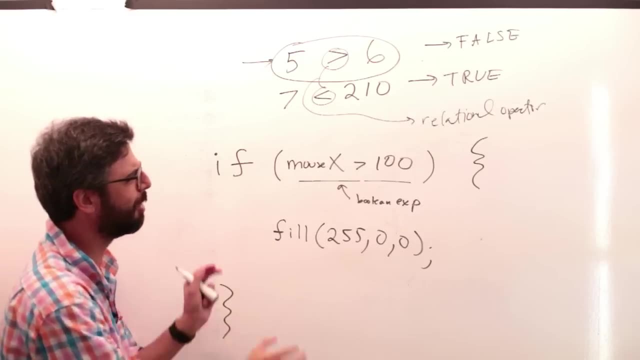 It will just sit there, never get executed. That's the power of a conditional statement. So let's go and look and put this into our example, and I think that will actually wrap up this video. just sort of the very, very basics, And there's more to it than this. 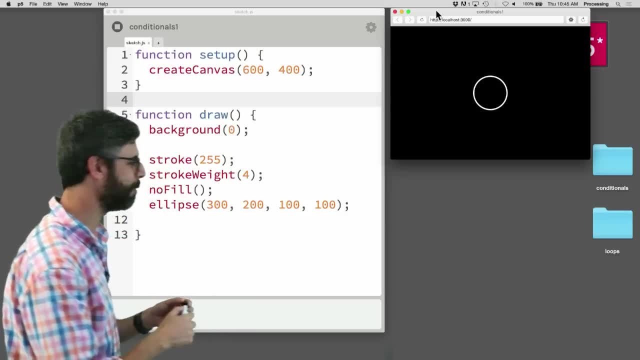 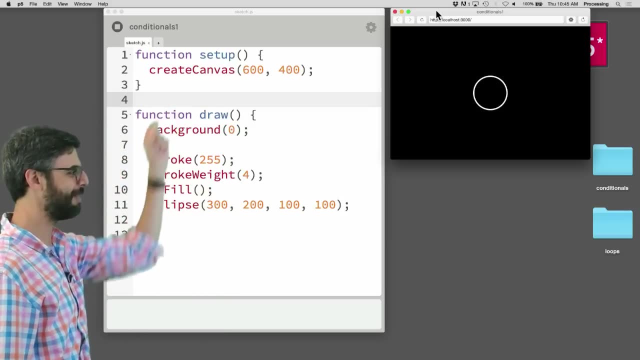 but I'll get to that later. Okay, so here we are. I have a nice simple example that I prepared in advance. This is me actually preparing to make one of these videos in advance. I've got createCanvas up here and I'm drawing a circle. 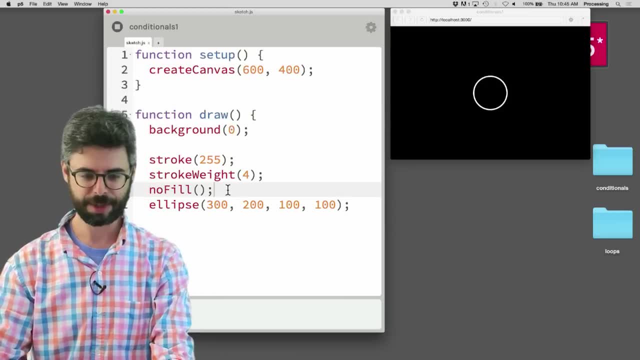 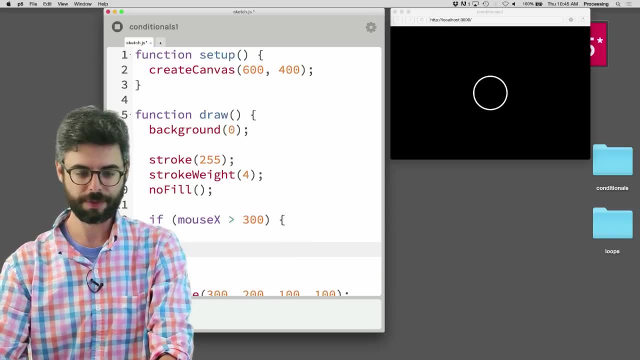 So no fill. What I'm going to do now is add something down here. If mouseX is greater than- and let's say 300, which is the middle of the window, fill 255.0,. let's try to give ourselves some purplish color. 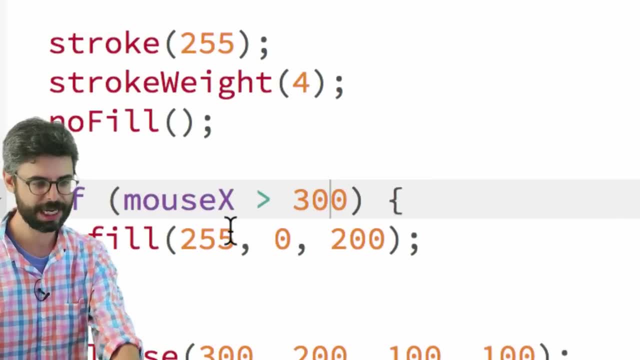 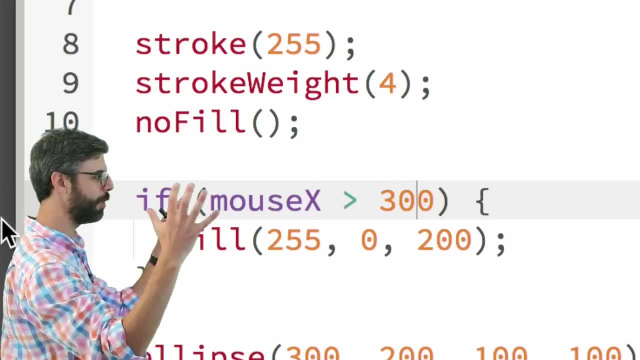 and we can see. this is what I've added here. This is the syntax, So you can see. whoops, let's move over here. You can see a couple things here. So the Boolean expression is in between parentheses. The if statement opens with a curly bracket. 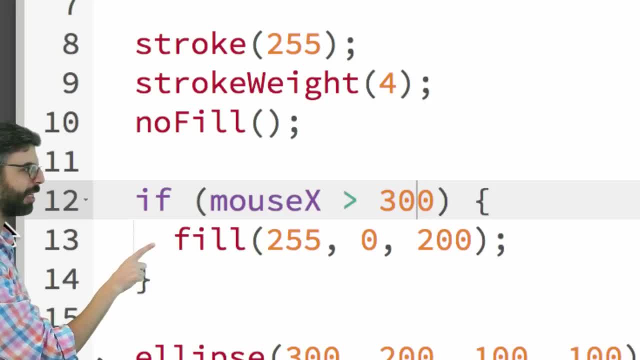 ends with a curly bracket, and notice how fill gets indented. So the indentation has not changed the way the code runs, but it helps you visually. see, You could have a lot of lines of code, you could have a lot of things happen. 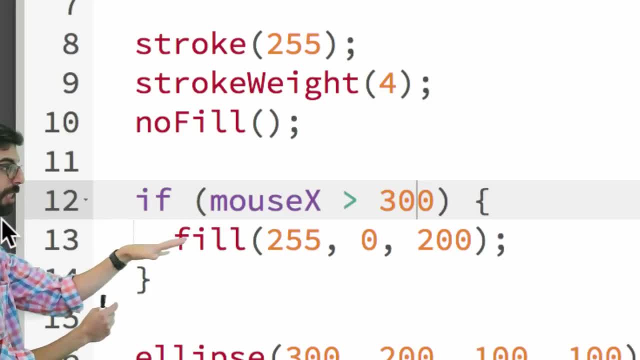 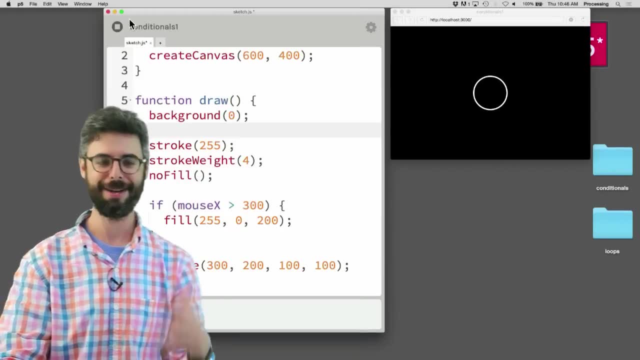 within that if statement, So those curly brackets say: this is the code that should be executed. And remember, if this evaluates to false, this doesn't happen, Draws looping over and over again. it might be true, it might not be true. 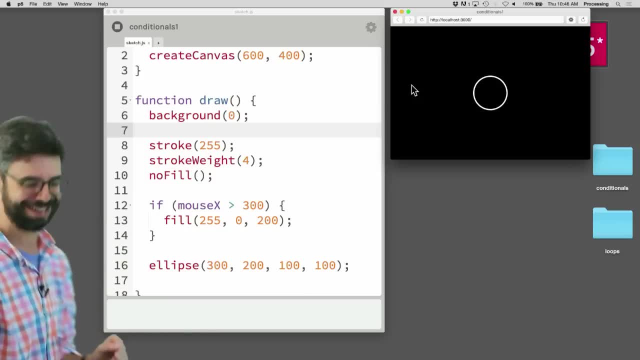 What's the mouse? I don't know. I think it's at like 50, so we're not there yet. Okay, it's like 100, 150, done 200.. Okay, we're getting there, we're close. 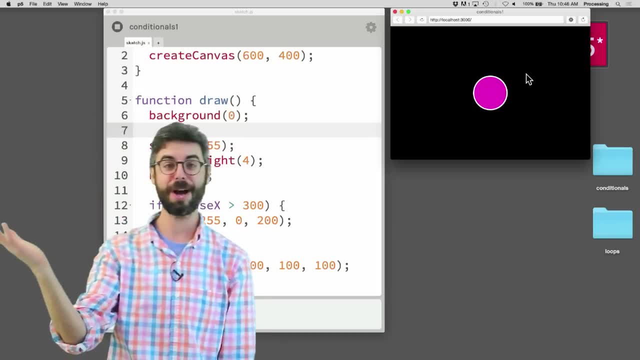 It's almost there. it's almost there. Oh, yes, we got it All right. so you can see that as the mouse gets beyond 300, that circle turns this purplish pinkish color. When I move the mouse back, it's off. 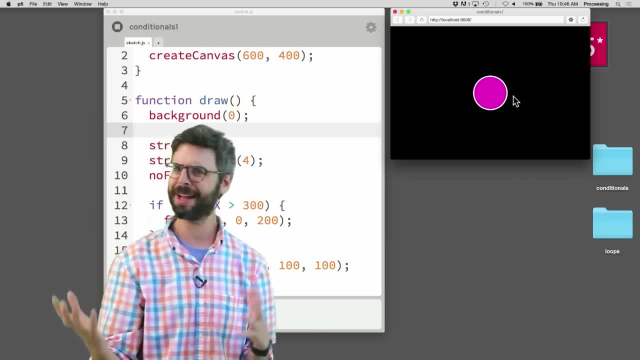 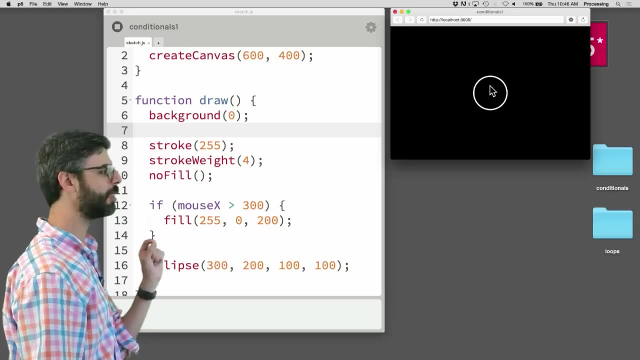 So this is pretty exciting and you could think, like, almost have this sense of like making a rollover here. I mean, we don't at all. what's that if? statement that says: if the mouse is inside the circle, highlight it. 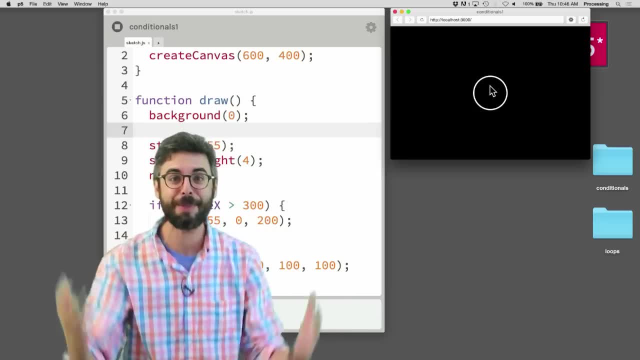 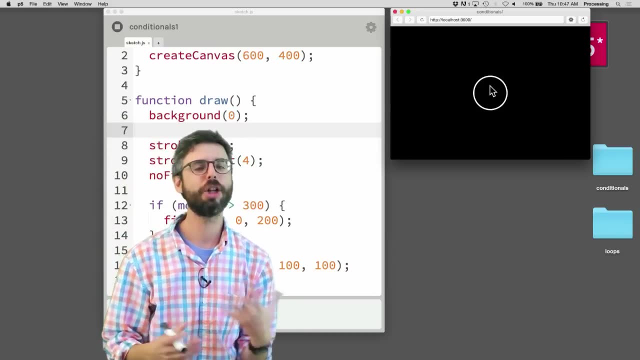 So these are the kinds of things, you know, all these interface elements that you might be used to using on your computer. this is how they work, And I don't know if I will actually solve this particular problem in a video. It involves looking up the distance function. 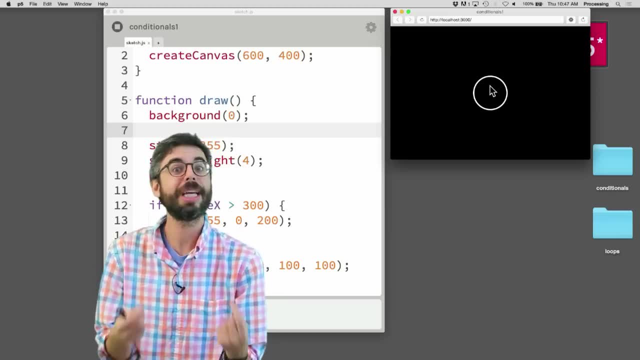 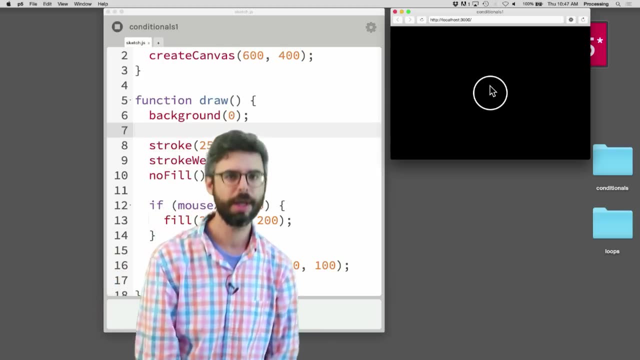 because you've got to test the distance of the mouse from the center of that circle. But that could be something. if you want a kind of tricky problem to look at, you might sort of see- Let's do an example that uses a rectangle. 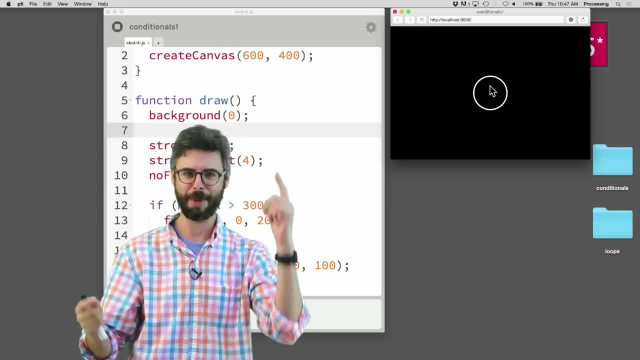 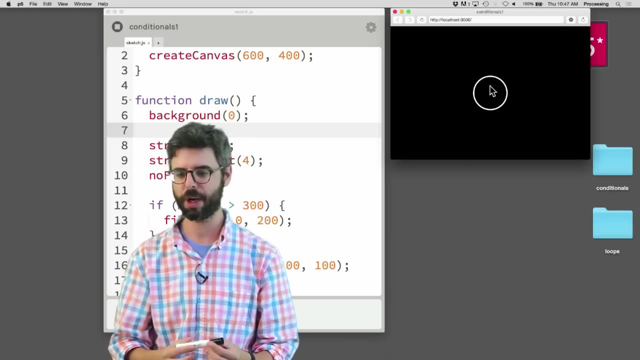 to try to see if the mouse is within the bounds of the rectangle. I think that's in my mind of future videos. So there's one other thing I want to mention, just to kind of like make sure this video kind of like wraps itself up. 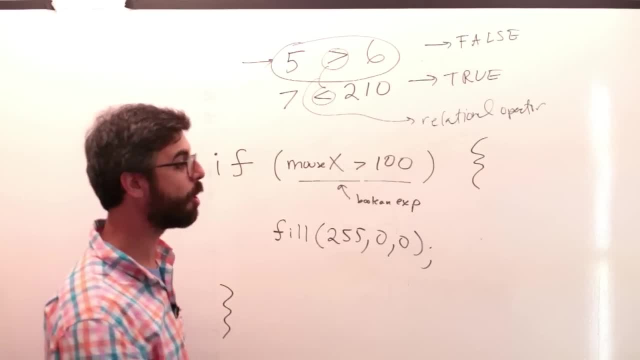 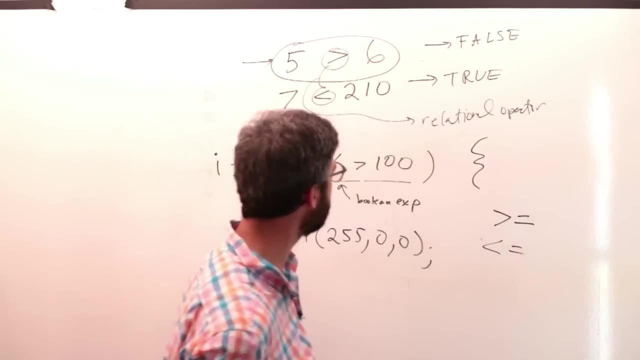 and doesn't leave off any details. I showed you these relational operators. There are other ones. There is greater than and equals. There is less than or equals. So in other words, 5 is greater than or equals 6. This is actually true. 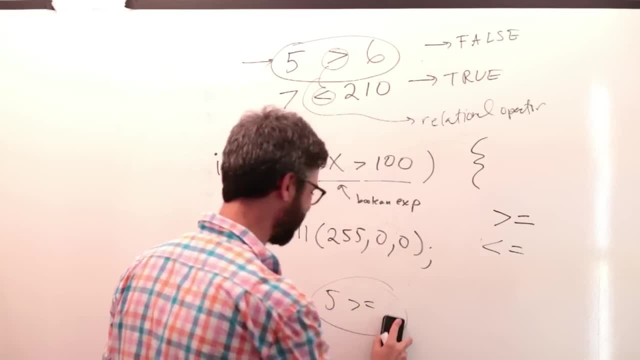 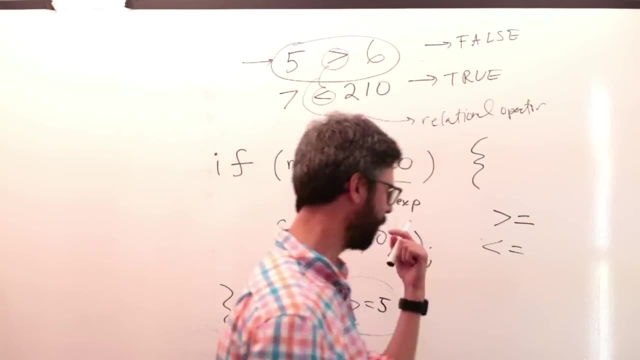 No, it's not. I meant to say like that's not true at all. 5 is greater than or equals 5, because it is equal. I was doing so well with this video. now I'm kind of losing my mind here a little bit. 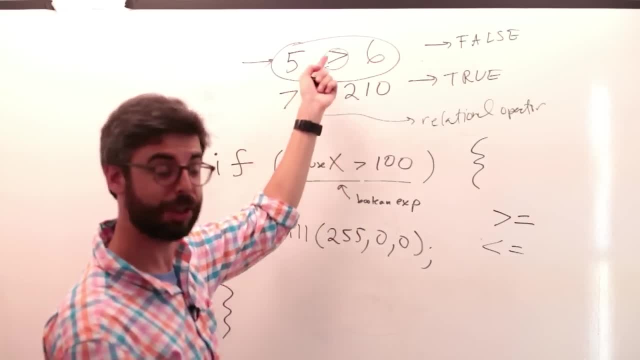 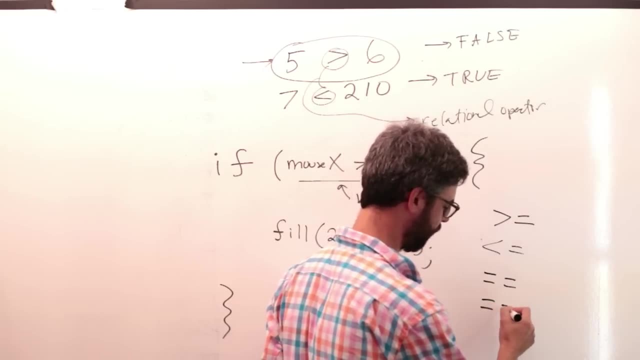 But there are other relational operators that you could use. These are probably the most common ones. you're going to get pretty far. And then there's also double equals. There's a funny distinction between the double equals and double equals in JavaScript that I'm going to leave out of this video.